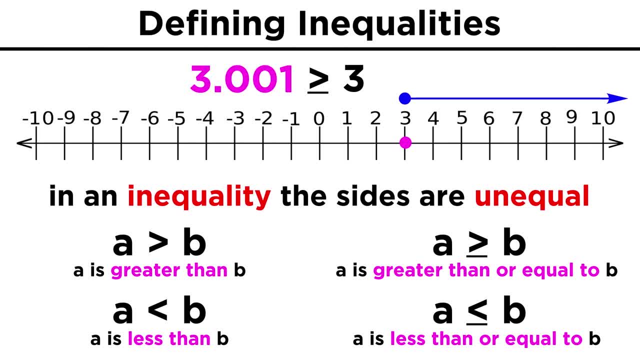 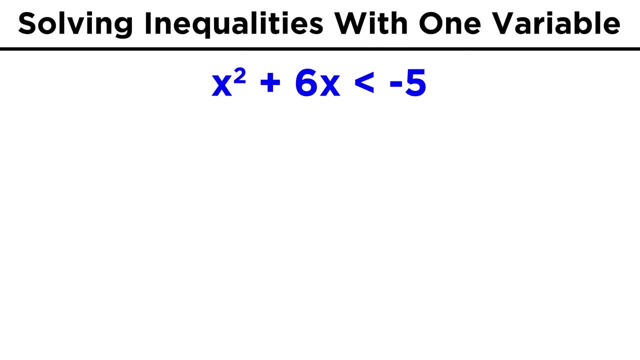 greater than three, including three. point zero, zero, one, pi, seven, halves or a billion. The first thing we need to do is learn how to solve inequalities that are a little more involved than the simple ones we've learned. Take something like X squared plus six, X is less than negative five. 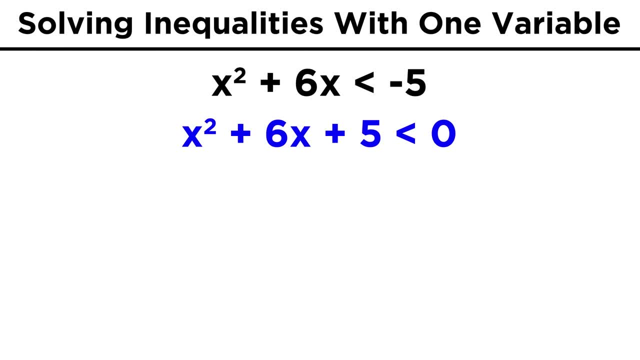 To solve this. we get everything on one side, so that the function is either greater than zero or less than zero. In this case, we add five and we get this. Then we pretend that the less than sign is an equals sign and we solve the equation. 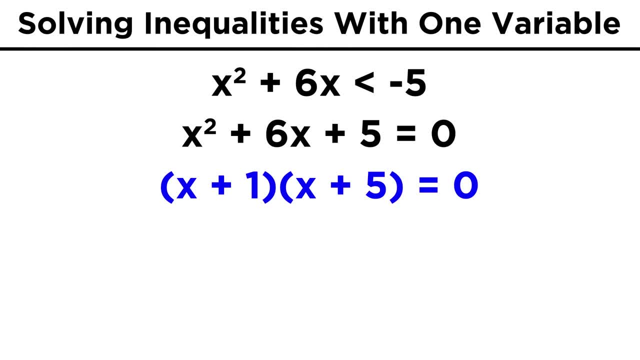 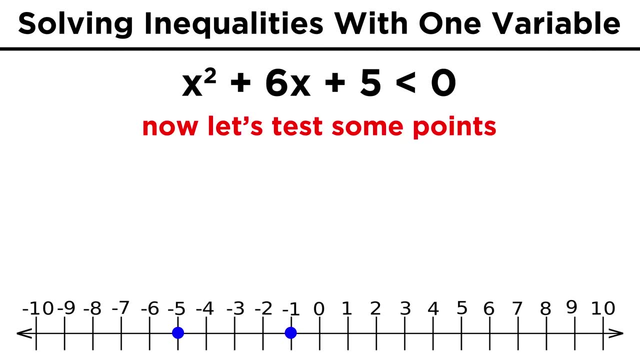 In this case that would require factoring this to get X plus one times X plus five, which gives us negative one and negative five as the solutions. Then we can draw a number line and mark these points. Then to see which sections of the number line satisfy the inequality, we just pick a point. 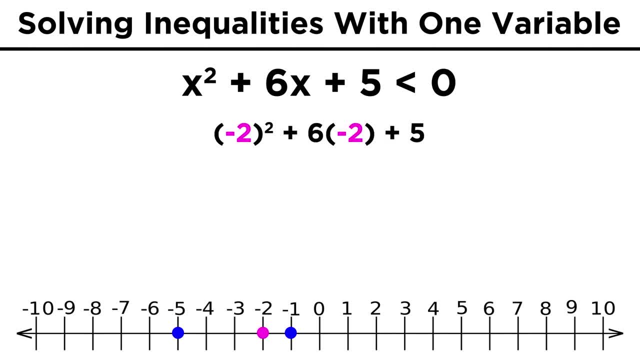 from each section and see if it works. In between. we could try: negative two. Negative two squared is four plus negative twelve is negative. eight plus five is negative three. Negative three is less than zero. So this section is a solution to the inequality. 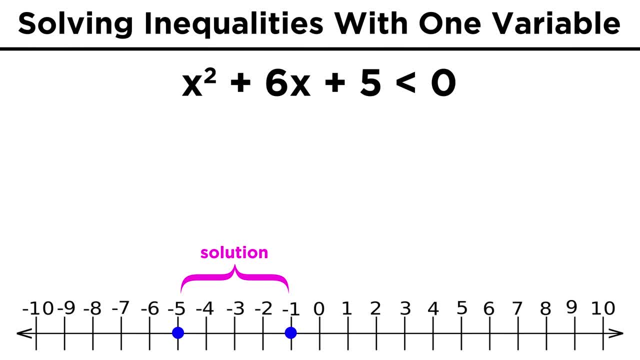 Now let's move over to the right. Zero is always an easy one to try, so let's use that. Zero plus zero plus five is five, which is not less than zero. so, from negative one to positive infinity, these values don't work. 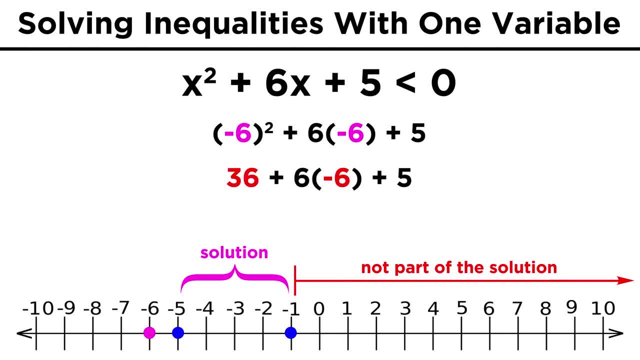 Trying the other side. let's use negative six. Thirty-six plus negative thirty-six gives us zero plus five is five, so none of these values work. The solution to the inequality is everything from negative five to negative one exclusive, which we denote by writing this parenthetical term. 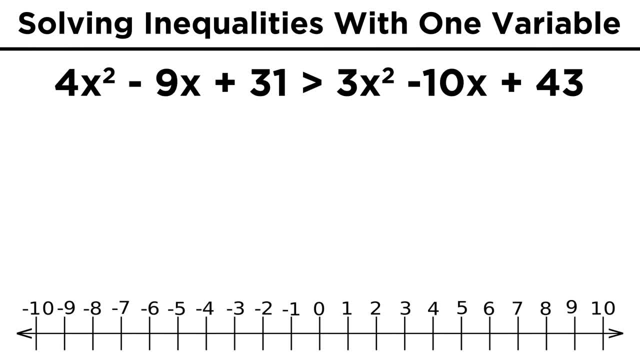 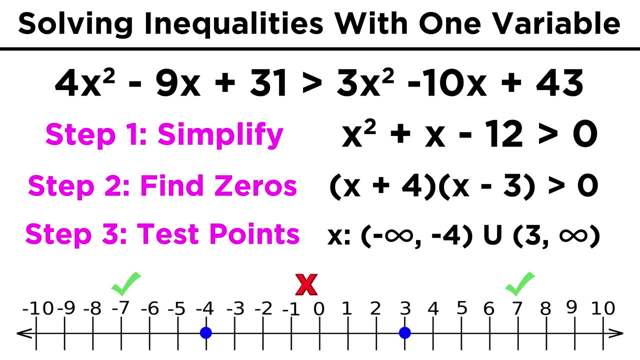 This approach will work for trickier inequalities with many terms on both sides. We just combine all the like terms on one side so that the other side is zero, and then solve Whatever the zeros are. we then just test points to find out which intervals make the 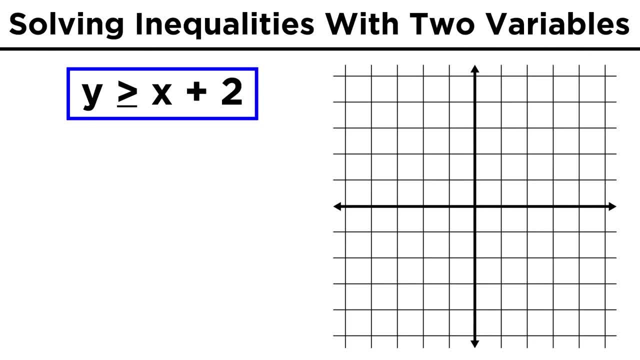 cut. When polynomial inequalities contain two variables, like Y is greater than or equal to X plus two, these become interesting to graph. When we do this, the first step is to treat this inequality as though it were an equation. so Y equals X plus two. 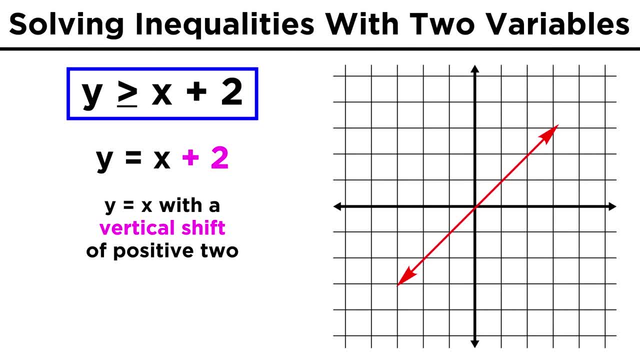 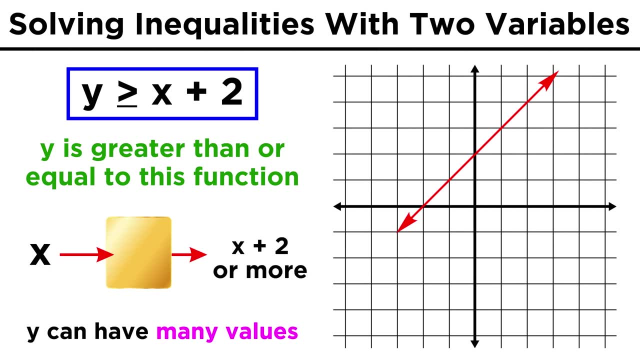 As we should know at this point, this will just be the line: Y equals X, but shifted up two, given this vertical shift term here. Now what the inequality says is that Y must be greater than or equal to this. So for any input X, Y must be greater by two or more. 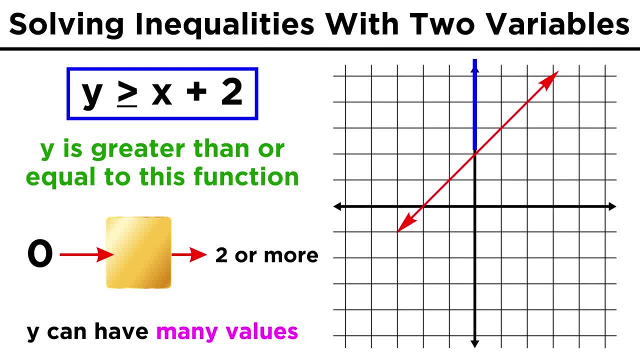 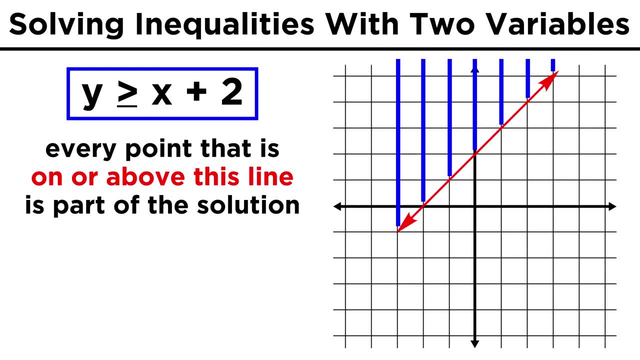 So when X is zero, Y must be two or more. When X is one, Y must be three or more. That means that every point on this line is a solution to the inequality, as is every point in the XY plane that is above this line. 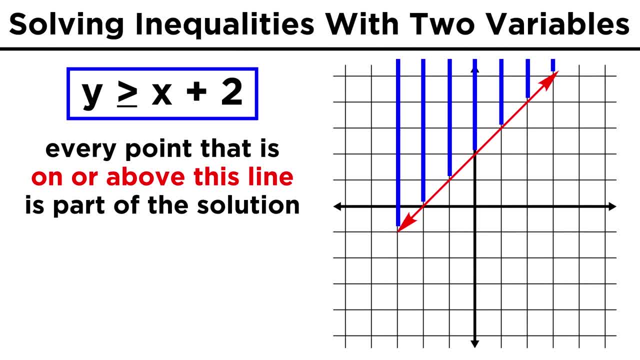 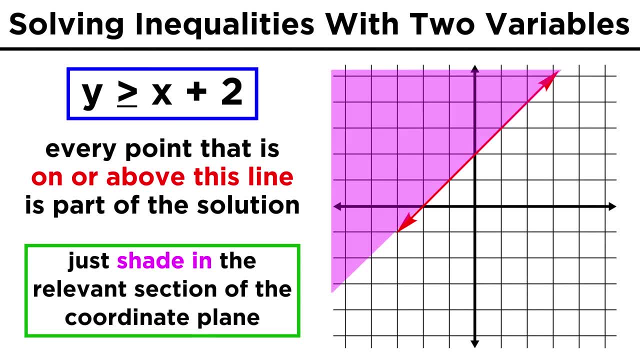 since every point above the line has a Y value that is greater than the corresponding Y value of the line. We would denote this by shading in this section of the coordinate plane, implying that everything above this line is a solution to the inequality. We can do the same thing for Y is greater than X squared minus four. 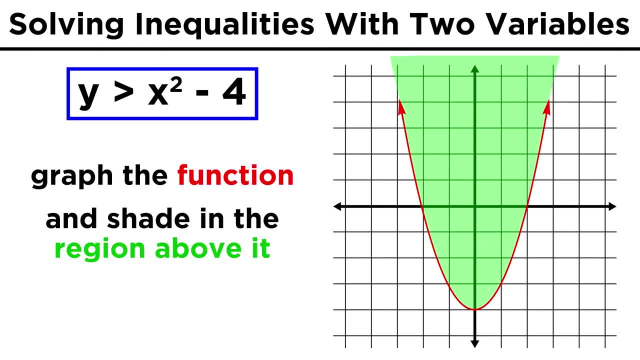 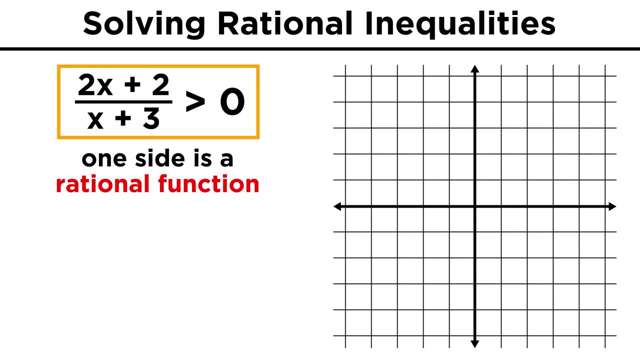 We just graph the function and shade in everything above it, or the section containing points with Y values that are greater than the Y value for the point on the function directly below. Now let's look at rational inequalities. As we could probably guess after learning how to graph rational functions, these are: 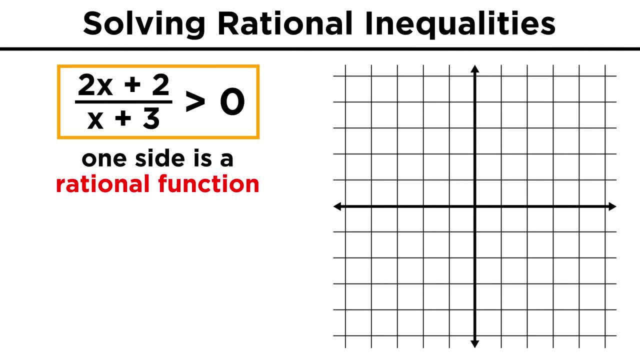 just inequalities. where one side is a rational function. Take something like two X plus two over X plus three is greater than zero. We can solve this by figuring out a few things about it. First, the X intercept. We get that by setting the function equal to zero. 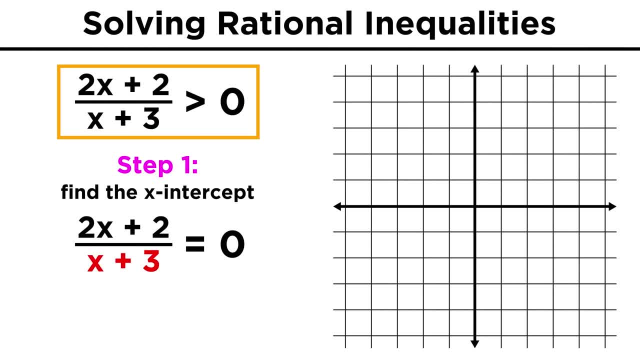 We can then multiply both sides by the denominator, which makes it vanish because when multiplied by zero it becomes zero. Subtract two divide by two, and negative one must be the X intercept. Then we can find the vertical asymptote by setting the denominator equal to zero.